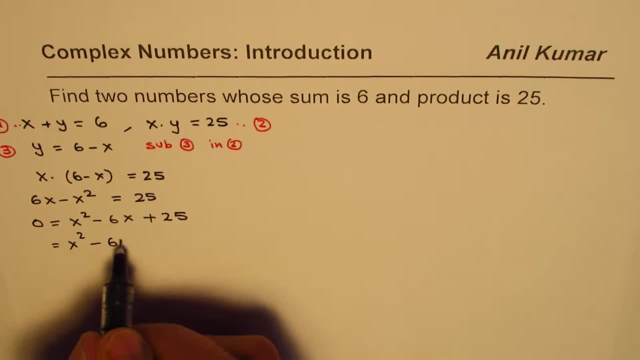 Subtitles by the Amaraorg community to complete squares. what should we do? we'll add and subtract square of half of 6, which is 3, right. so we'll add and subtract 3 square. this is completing the squares method. we could have used quadratic formula also to find the solution now here. this could be written as x minus 3, right. 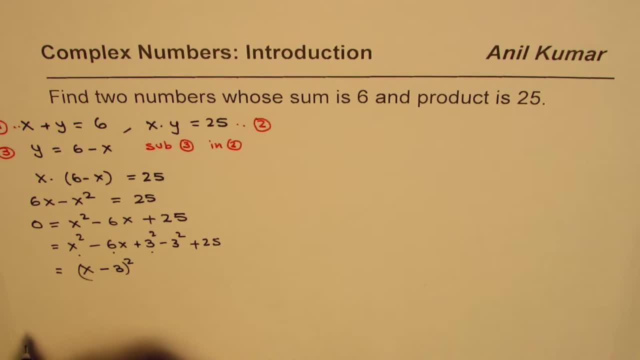 whole square, since first three terms form a perfect square. then we have minus 9 plus 25, and that gives us x minus 3. whole squared minus 9 plus 25 is plus 16, right, so that's what we get: 0 equals to this. now to solve for x, we'll take 16 on the left side. all this is 0, right. 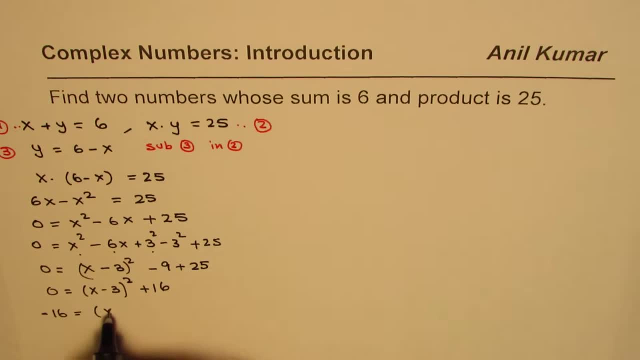 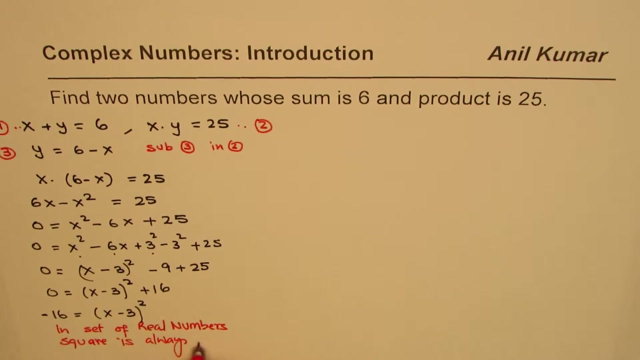 so we get minus 16 equals to x minus 3 whole square. now, at this stage, earlier, we kind of stopped. stopped Since we know in set of real numbers square is always positive, never negative, Square is always positive, And so we said no solution. So when we were talking about 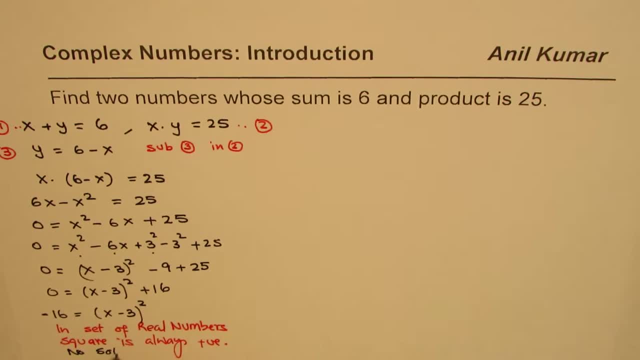 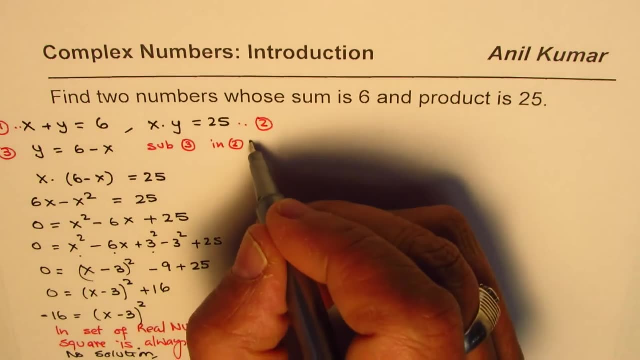 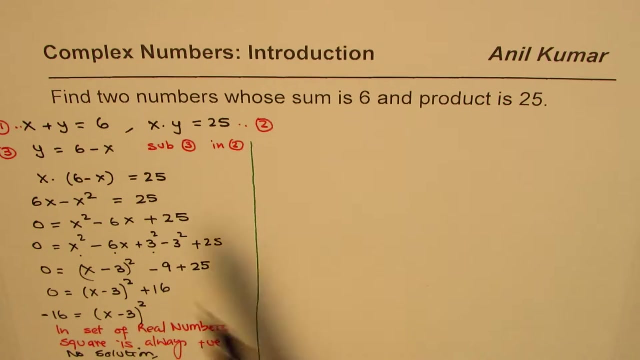 real numbers. we said no solution, Correct. So that is the place where we stopped and kind of gave up. Now let us continue from here and try to find a solution and see whether our conditions are met or not. So we will again continue from here. What we are writing: 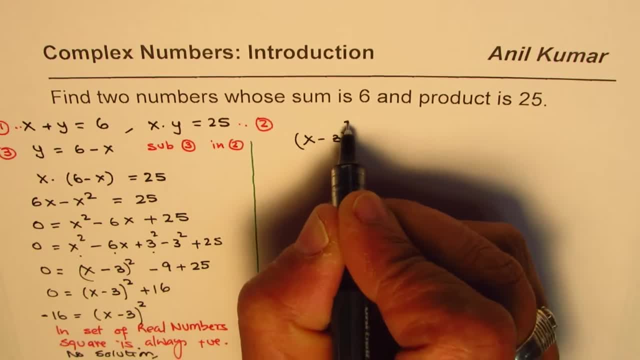 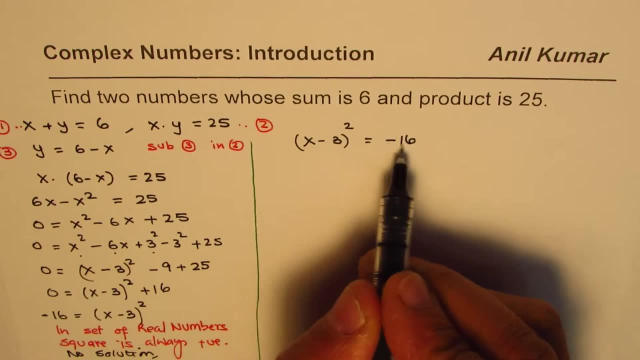 is we are saying: x minus 3, whole square equals to minus 16, okay, Now let me continue with minus 16.. What do I get? I get: x minus 3 equals to square root of minus 16.. And whenever you do square root, you get plus and minus. And then we can say: 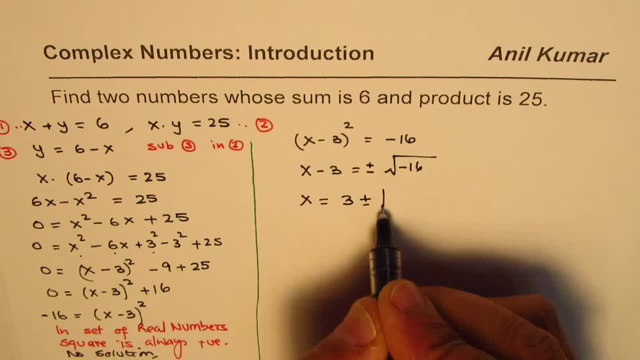 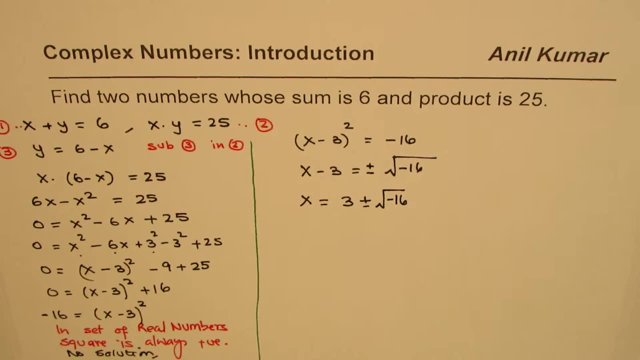 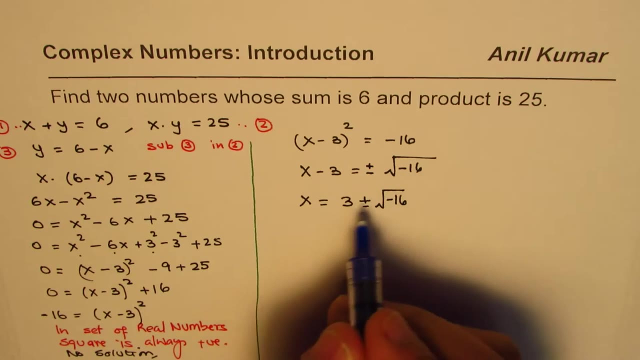 x is equals to 3 plus and minus square root of minus 16.. So that is what we get. Now we are saying that the solution of the question which we began with, that is, square root is sum is 6 and product is 25, is kind of like this. So that means we got two numbers here. 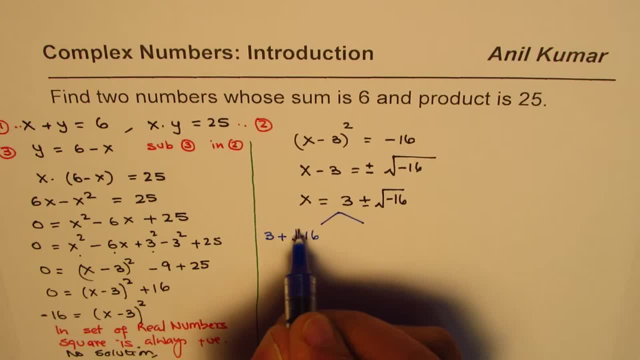 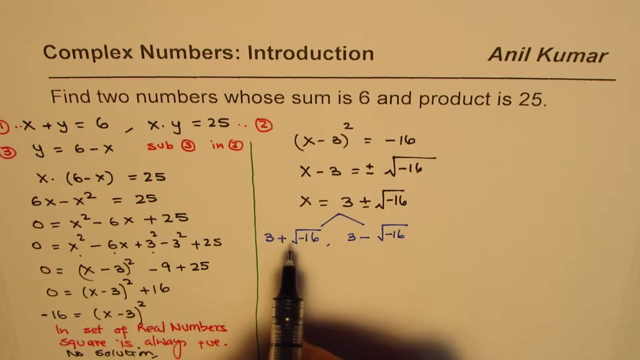 One is 3 plus square root of minus 16 and the other one is 3 minus square root of minus 16, correct. Now, in the set of real numbers this does not make sense, but let us see what happens if we add these two. okay, Let me add these two. If I add 3 plus square root. 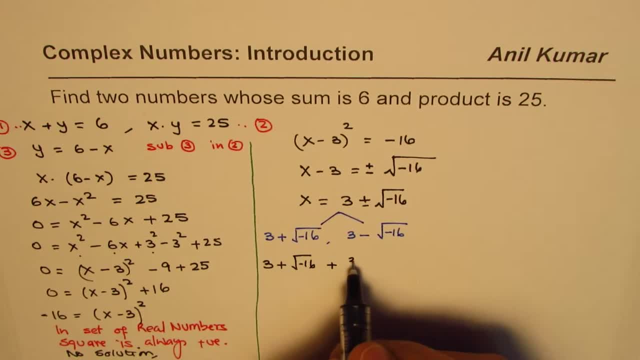 of minus 16.. Plus 3, minus square root of minus 16.. What do I get Now? these two terms cancel out, right? So these two terms with plus and minus cancel out, And what you really get is equal to 3 plus 3, which is 6, right, So we did get sum of 6.. Do you see that? Sum of 6, correct. 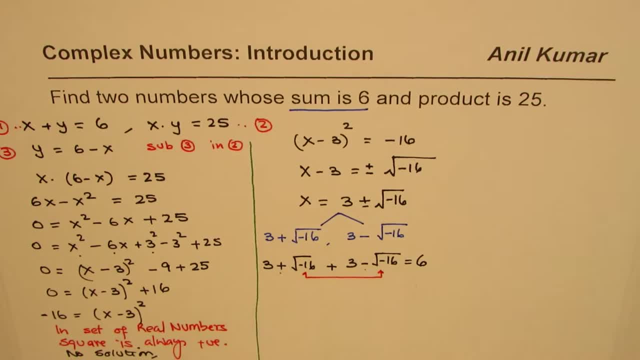 Now let me multiply these numbers. Let me multiply these numbers and see what do I get. So now we have 3 plus square root of minus 16 times 3 minus square root of minus 16.. So when I multiply, I get 3 times 3 is 9, and then I get minus 3 square root of minus. 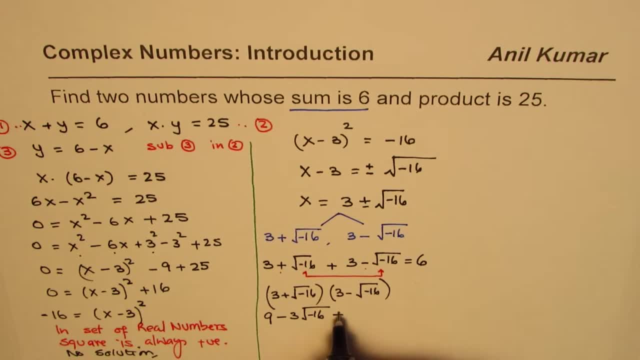 16. And then with this I get plus 3 times square root of minus 16. And when I multiply this part kind of, I get Square root of minus 16 square right. So this is kind of tricky, but what we really 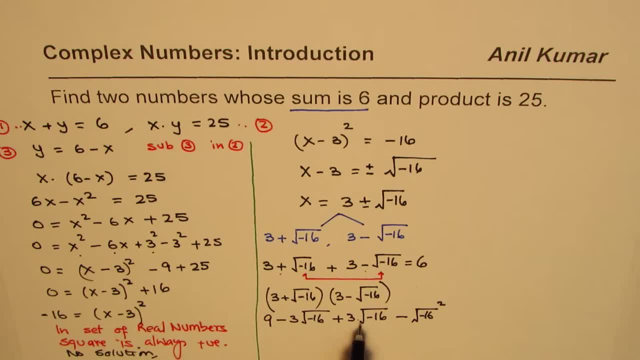 get here is that these two cancel out, right. And here we get 9 minus Now square of minus 16,. I mean because, assuming that we could write this as 16, right, so assuming square root of this number, we could write it as such. what I'm trying to say is, if you 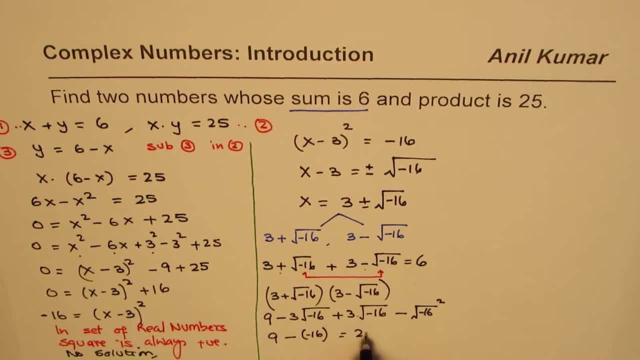 write this as minus 16, then we do get 25. do you see that? I'm not saying this is the correct step, but what I'm trying to say here is that we could get 25 if somehow we could have written this number as this, but I mean to say square of this number- as negative 16. right, then we could have. 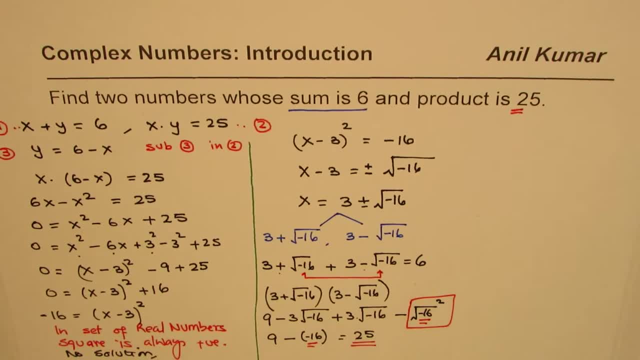 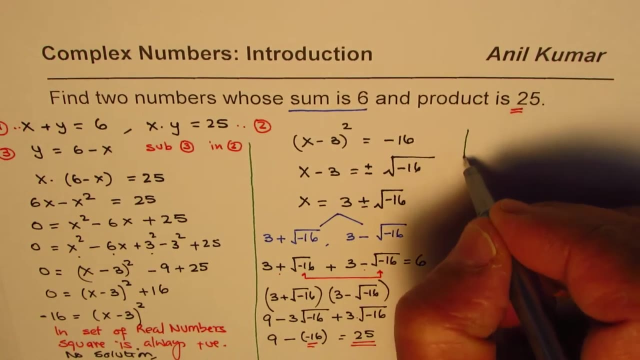 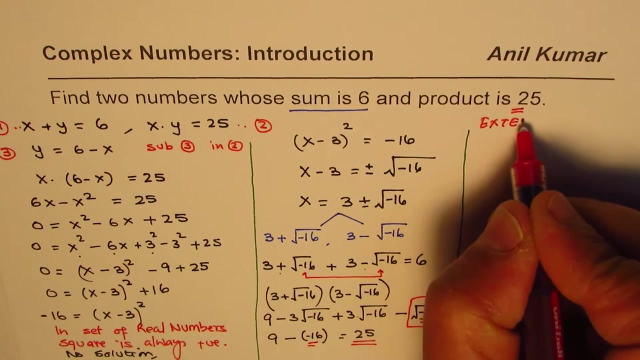 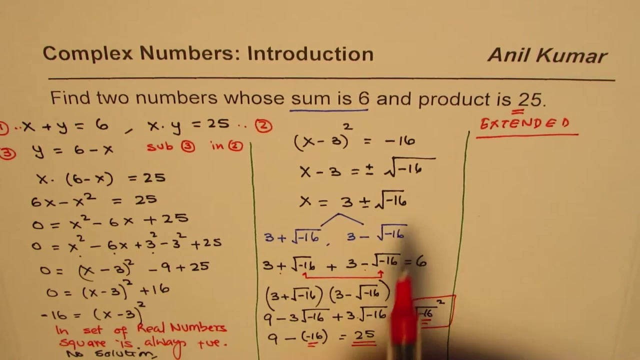 got that result also right. so that gives kind of an idea that this result which we got was not really absurd, right, it could make sense if we could extend our number system, right? so so what, logically, mathematicians did that? they extended the mathematical set of numbers to include another number, so that we 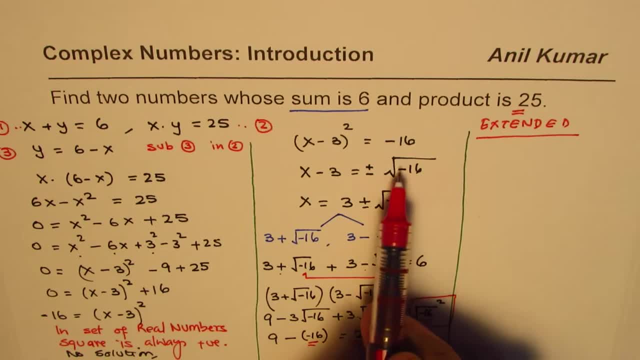 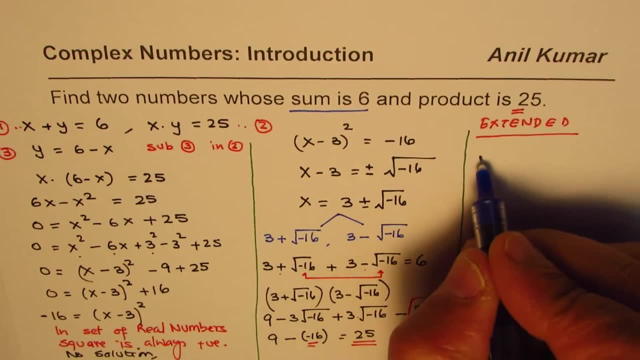 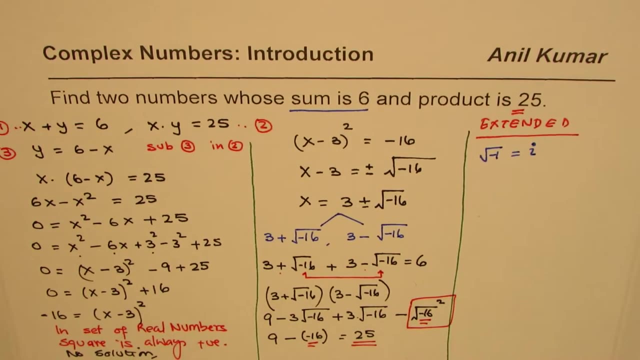 could also solve equations where we have negative within the square root, right. and then they said: well, let us say that square root of minus 1 is some imaginary number- that is what I is- imaginary number- and then if we could get the square root of this number as negative 16, right. then we could have 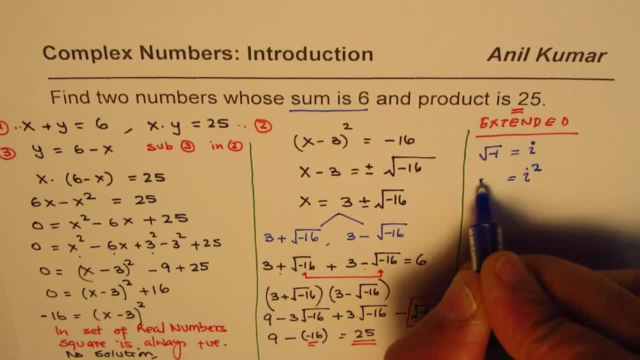 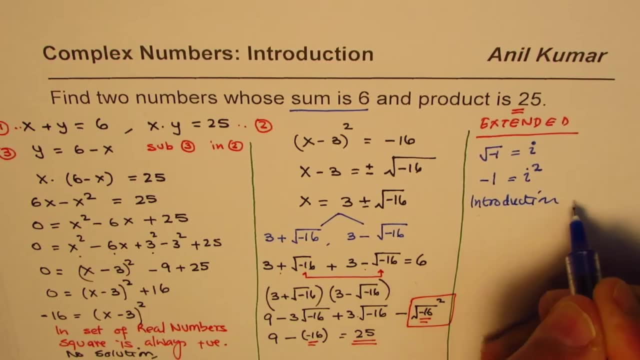 that result also right. so what I'm trying to say here is that if you could have got that result also, that case square of this imaginary number will be minus 1, right. So that is kind of introduction of imaginary number, which was given the sign i for imaginary We call it. 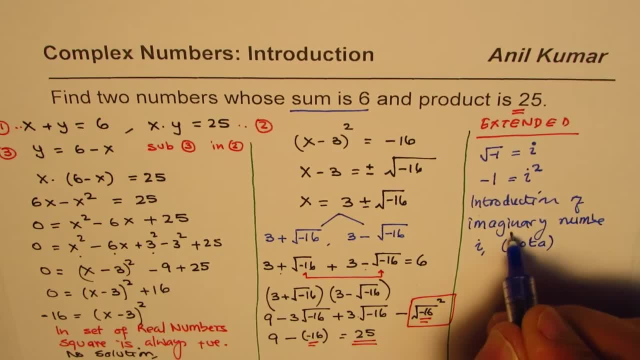 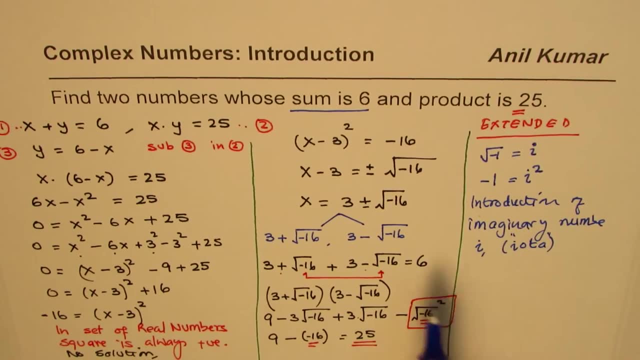 when we say iota, we call it iota, a Greek symbol, iota right. So that will be the symbol being used. So now in the set of complex numbers. so this is imaginary, so this set was called set of complex numbers. okay, So now in the set of complex numbers, we 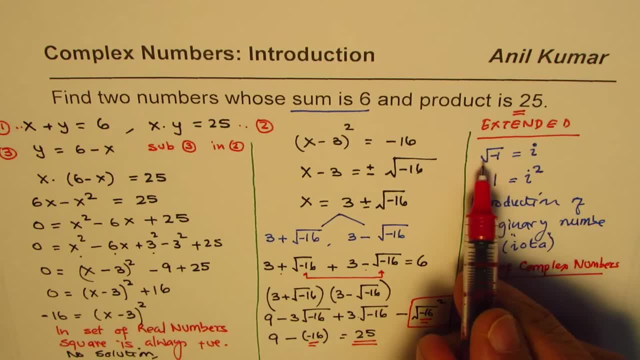 have all the real numbers, plus such numbers which have square Square root of minus 1 also included. Now, taking the set of complex numbers, we could actually provide the solution for this one right. So this now, all of a sudden, has a. 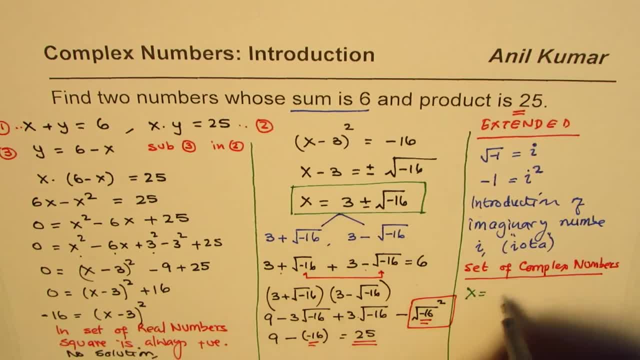 lot of meaning. We could write x as equals to 3 plus or minus. So we are saying square root of minus 1, is i right? So you can say i and what is square root of 16?? It is 4,. 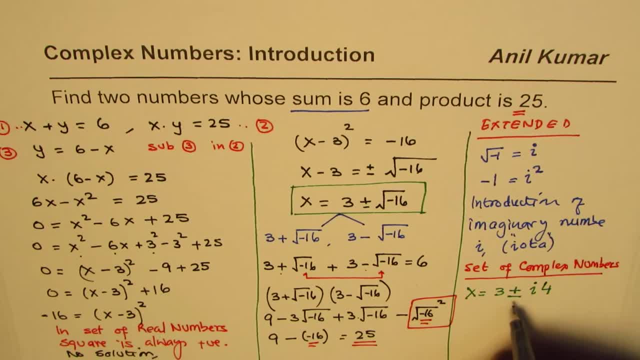 right. So it is 4.. So we could write this as Kansas Real and complex part. So in this case is good to normally right this as x plus minus 4 i. So we say we have two solution here. one is x plus 4 i, the other one is x.